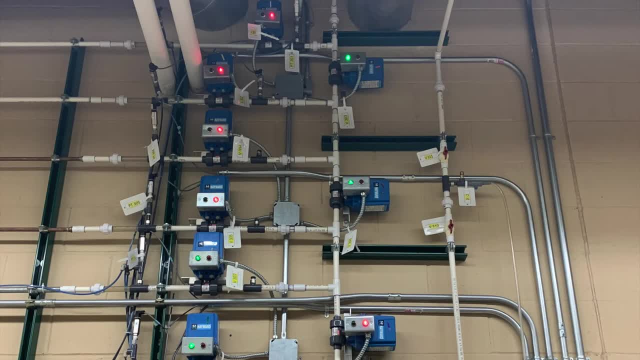 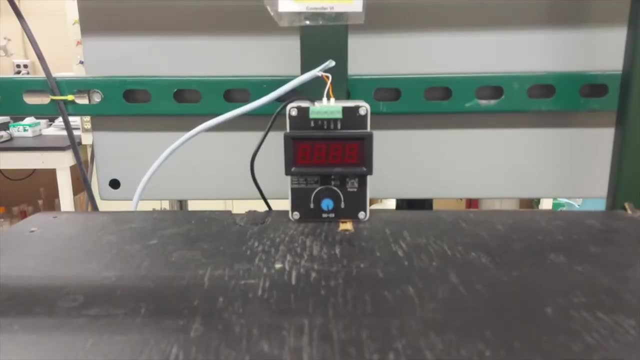 here is the proper pathway for the copper pipe And here is the one for the ductile iron pipe. Once your loop is set up, it is time to open the main valve. In order to operate the pump valve, we will be using this control box. 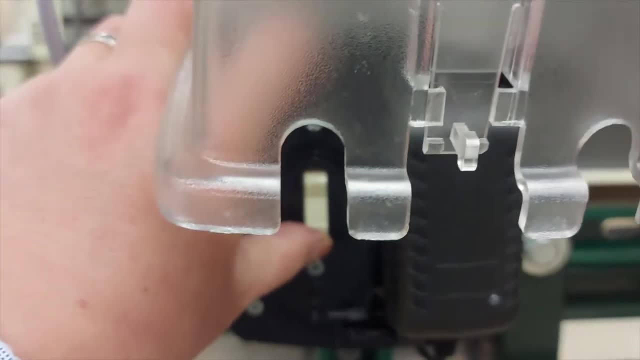 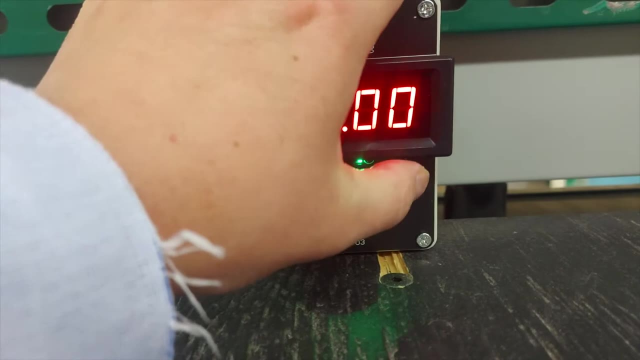 To begin. turn on this switch so that the valve actuator's blue LED light turns on. This also results in the control box's display turning on. If the green LED light is on, press the display button to switch it to red so that the control 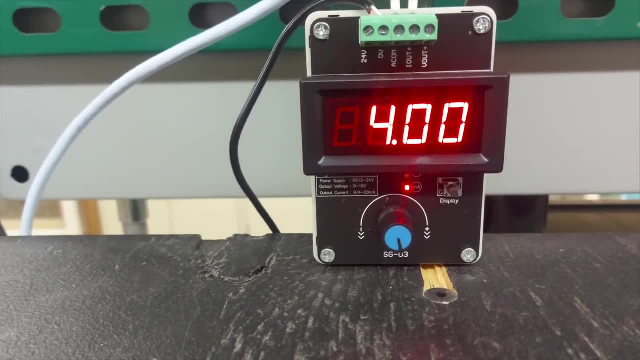 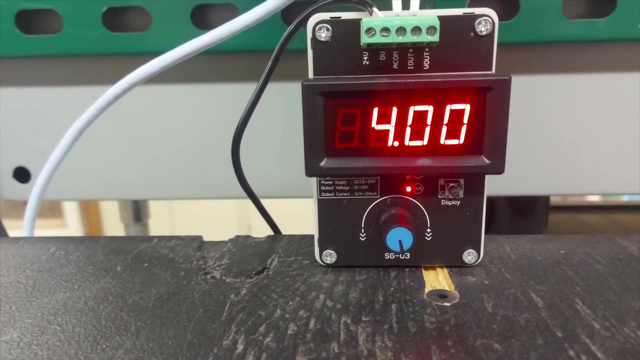 box is in milliamps. The lowest value for the control box on this setting is 4 milliamps, which corresponds with the valve being completely closed. The current generator has a range between 4 and 20 milliamps with a linear relationship. 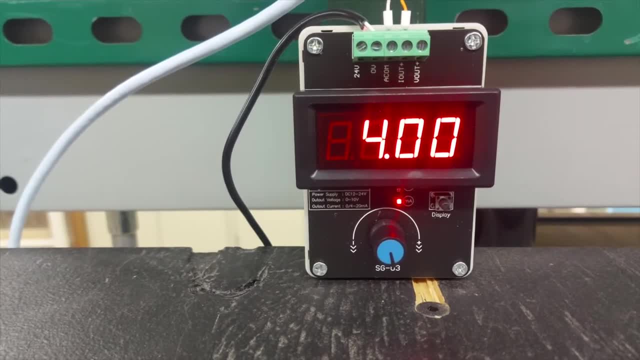 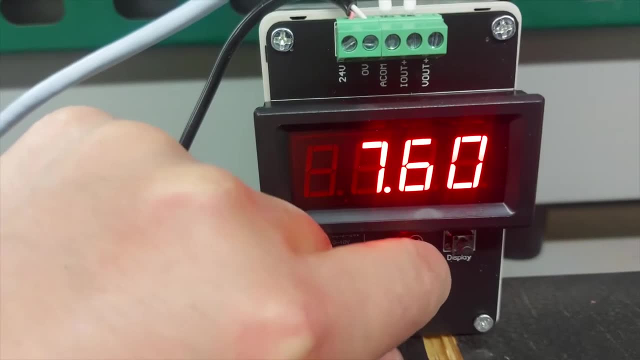 between milliamps and the percent opening of the valve. For example, when the control box is set to 6 milliamps, the valve opens 12.5%. When the control box is set to 8 milliamps, the valve is 25% open. 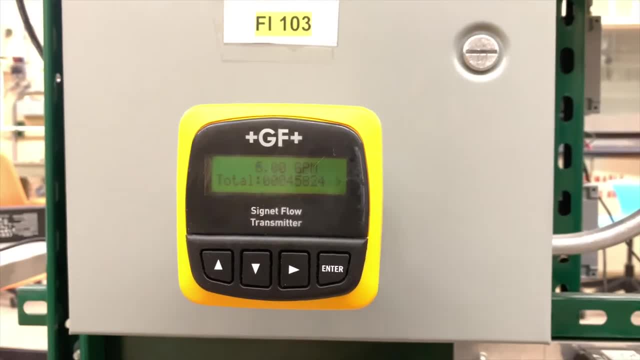 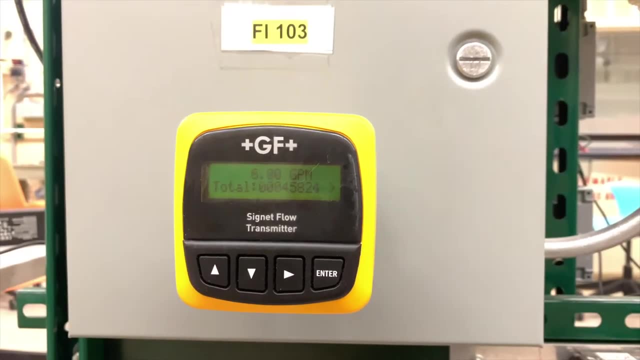 You will need to take three flow rates for each pipe. Firstly, increase the control box values incrementally, recording the corresponding flow rates. Then select three flow rates well spaced from one another, so that you have a low flow rate, a medium flow rate and a high. 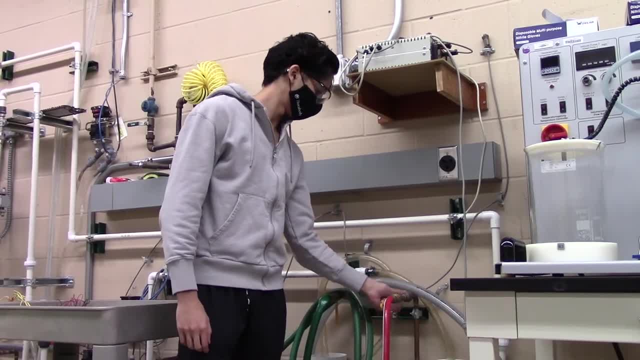 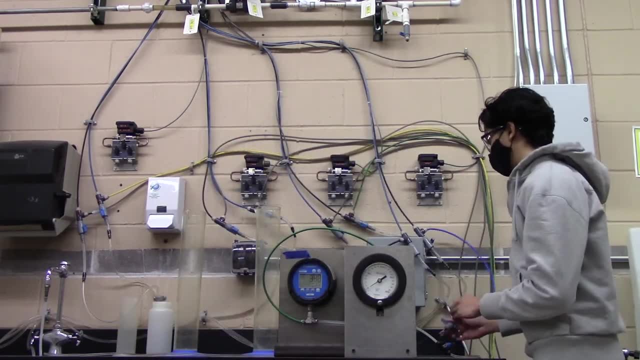 flow rate. You may then open up the main water valve. Once you have set up your system to your desired flow rate, you may now take your pressure readings. To do so, you must find the three-way valve associated with whichever material you are working with. 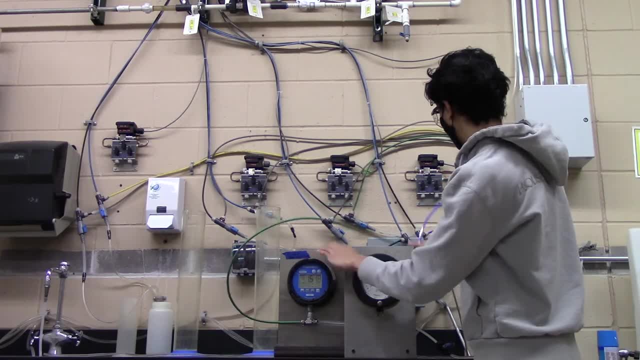 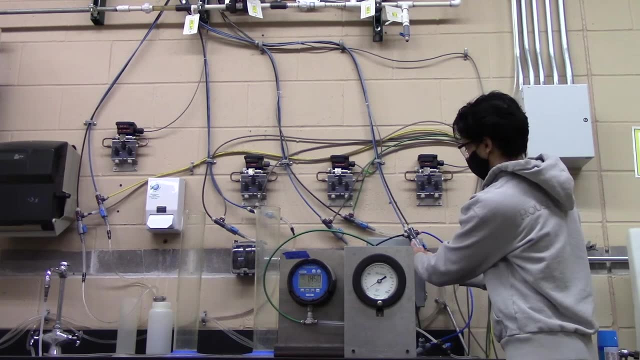 You then must connect this three-way valve to the pressure gauge To remove any excess air out of the system. you must bleed out your material's valve for at least 30 seconds. Once you are done bleeding and your valves are closed, once more, you must bleed out the. 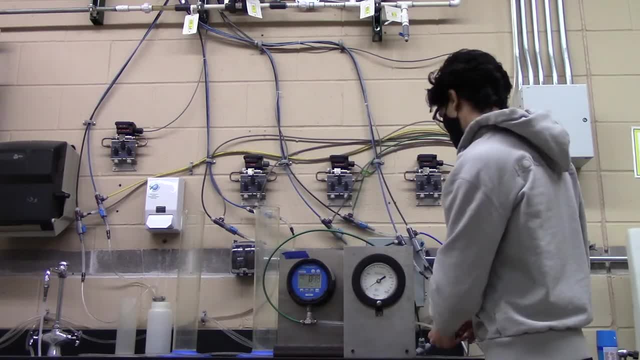 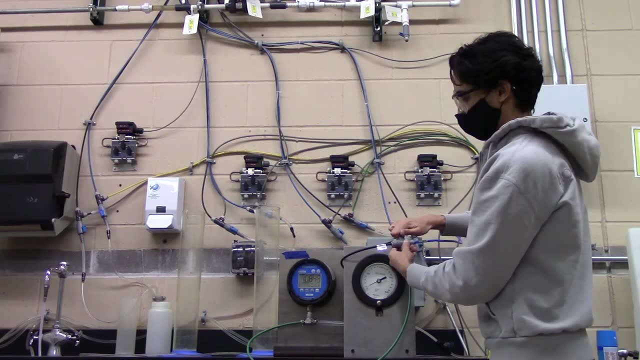 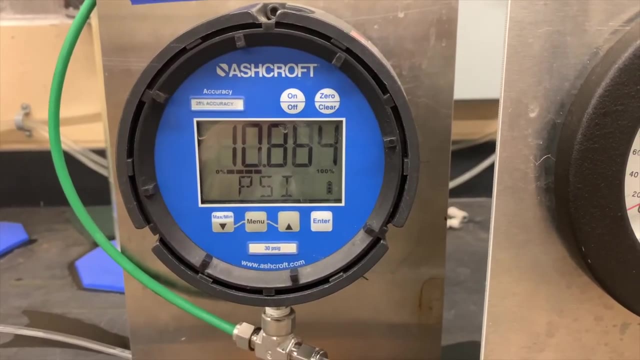 pressure gauge's valve again for 30 seconds. Then take your three-way valve connected to the pressure gauge. turn the valve to one side to get one pressure reading and the other side to get your second pressure reading. Higher pressure reading accounts for your initial pressure, while your lower pressure